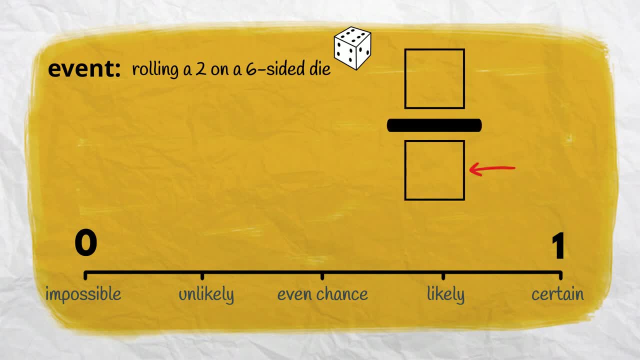 Within the fraction, the denominator shows the total number of possible outcomes in our event, In the case of probability. In the case of our event, the possible outcomes are rolling: a 1, a 2, a 3, a 4, a 5 or a 6.. 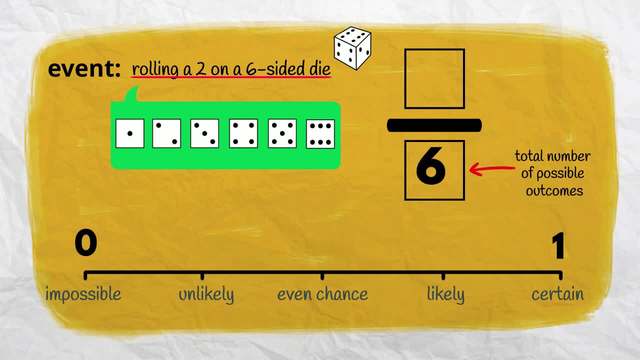 There are 6 possible outcomes, so our denominator is 6.. The numerator, the number at the top, shows the number of ways the event can happen. In this case, there is only one possible way: our event can happen by rolling a 2.. 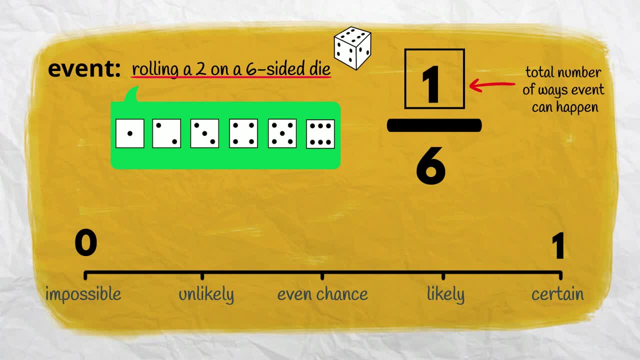 So our numerator is 1.. The probability of rolling a 2 on a 6-sided die is 1 in 6.. We can represent this as a decimal by calculating 1 divided by 6.. 1 divided by 6 is 0.166 recurring. 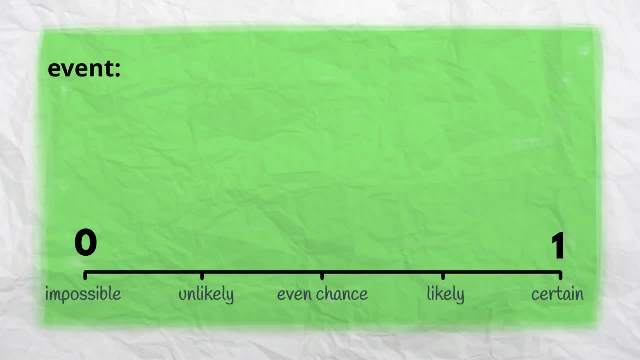 Let's now calculate the chance of a new event, this time rolling an even number on a 6-sided die. Let's start with the denominator: What are the total number of possible outcomes? Again, we could roll a 1,, a 2,, a 3,, a 4,, a 5 or a 6.. 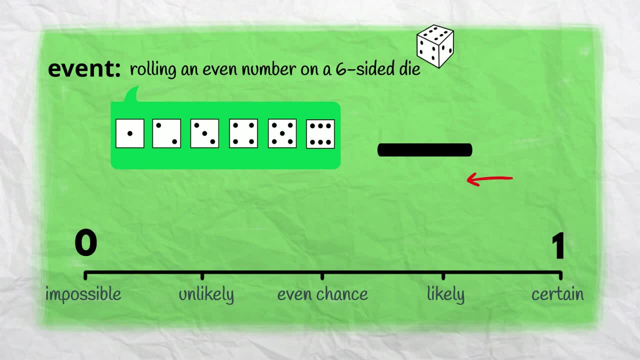 There are 6 possible outcomes. so again, our denominator is 6.. Now for the numerator. How many ways could our event happen? If we roll a 2, our event has happened, The same as if we roll a 4.. Or if we roll a 6.. 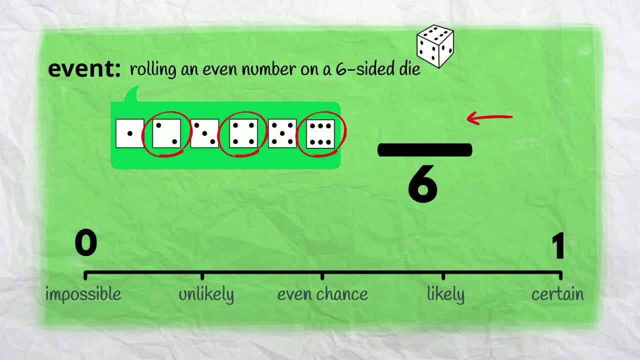 There are 3 ways our event could happen. Our numerator is 3.. The chance of rolling an even number is 3 in 6.. Simplifying this fraction, we get 1 in 2, an even chance. 1 divided by 2 is 0.5.. 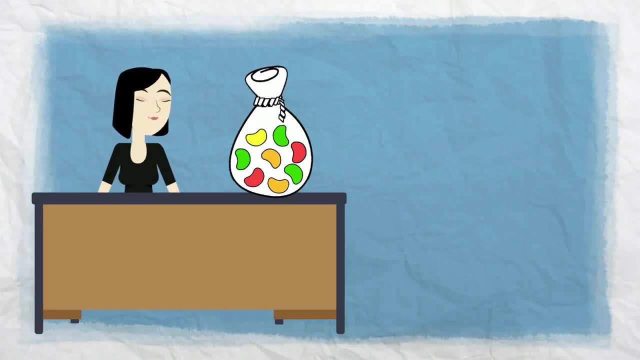 Let's now consider a new scenario. Imagine closing your eyes and choosing a jelly bean from this bag. Calculate the chance of picking out a yellow jelly bean, a green jelly bean, a jelly bean that is not red, a green or an orange jelly bean, a blue jelly bean.